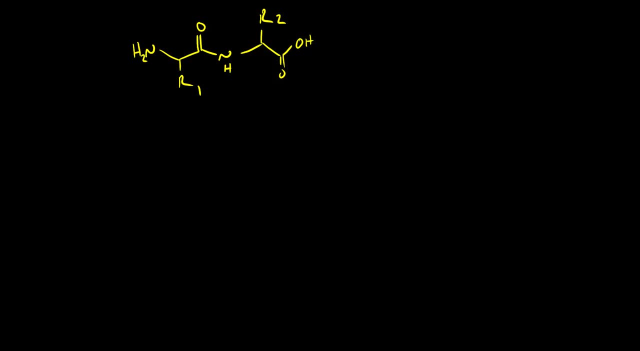 important part of drawing peptides correctly. Okay, so the first thing you need to do is to draw an NH2 group. Right, we call this the N-terminus. This is the part of the polypeptide where we have a free amine. 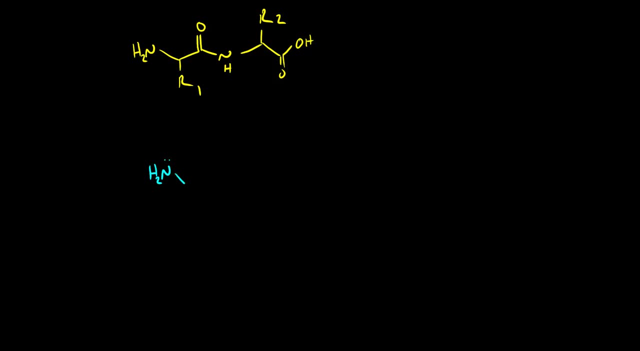 And then from the NH2 group, we have an alpha carbon, we have a carbonyl, We now form our peptide bond. Okay, so far we've got nitrogen, alpha carbon, carbonyl, next nitrogen in the peptide bond. Next we go to another alpha carbon and then to a. 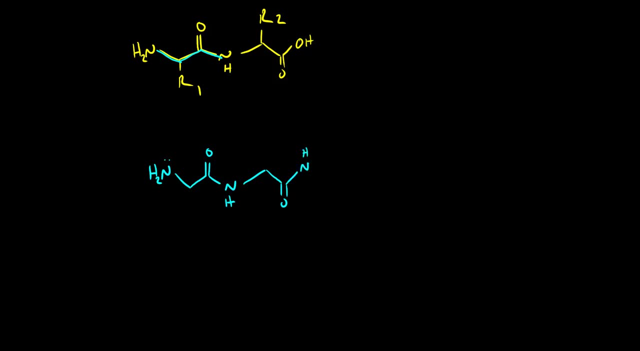 carbonyl. and then we make our peptide bond with another nitrogen- Alpha carbon carbonyl Nitrogen- alpha carbon carbonyl nitrogen- alpha carbon carbonyl nitrogen. So this theme keeps going and going until you reach what we call the C-terminus, which 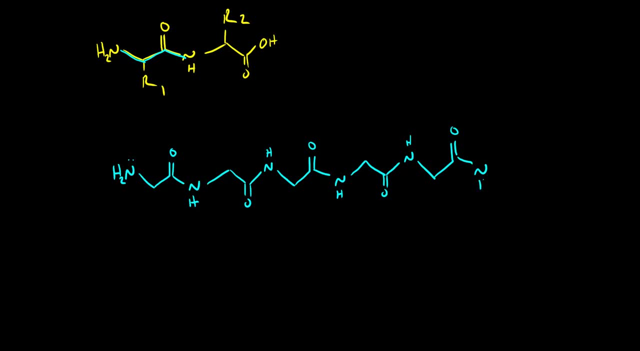 is the carboxylic acid end of our peptide, So I'll draw one more here. So instead of now making a peptide bond, we're going to go ahead and draw in the carboxylic acid. So this is a proper peptide backbone. 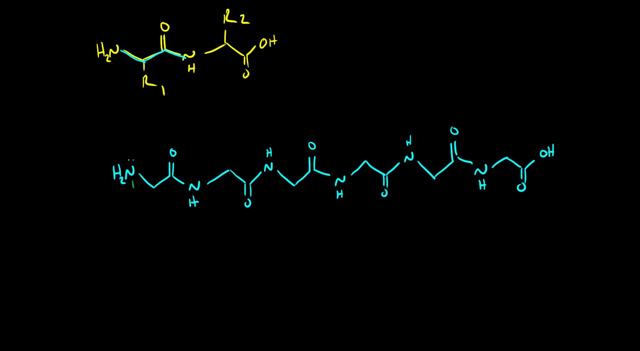 Every single linkage is a repeating pattern of nitrogen alpha carbon carbonyl. nitrogen alpha carbon carbonyl. nitrogen alpha carbon carbonyl. If you don't see this repeating pattern, you have not drawn it correctly. 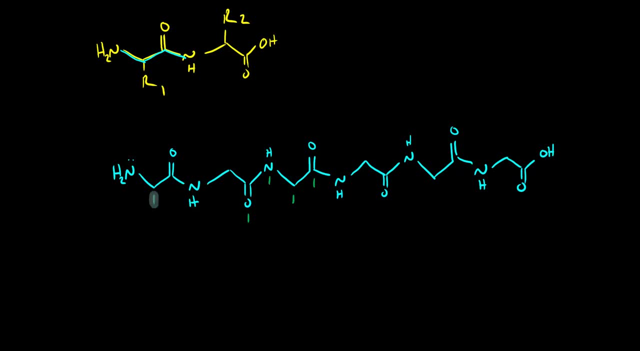 So we know that. We know that each alpha carbon then has an R group or a side chain hanging off of it. So this would be R1. We call this R2. This R3. And it's only when you start adding in the side chains that the actual amino acid matters. 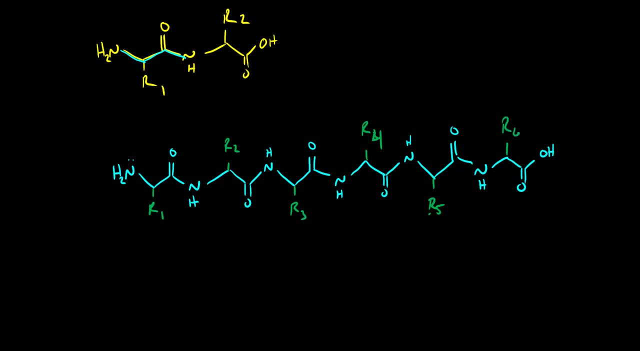 Before you start putting in the side chain, when all you're doing is focusing on the backbone, it doesn't matter what these side chains are. It's only when you determine What the amino acids are where the side chains matter. So let's go ahead and give this a shot. 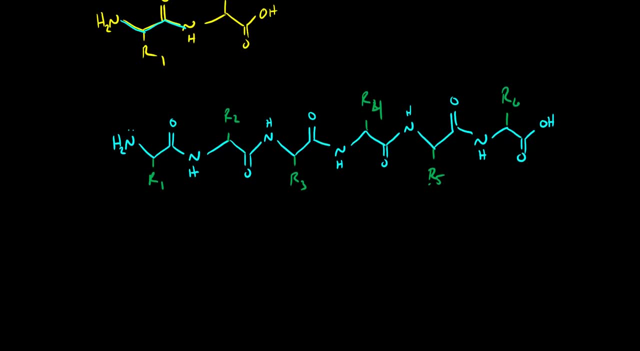 Let's say that we want to draw a polypeptide that has the sequence Asp. Alla Lys. You may remember the three letter abbreviations. If you don't, please become familiar with them. So Asp is aspartic acid. 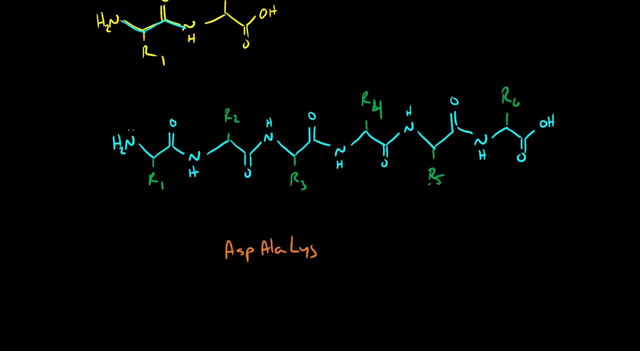 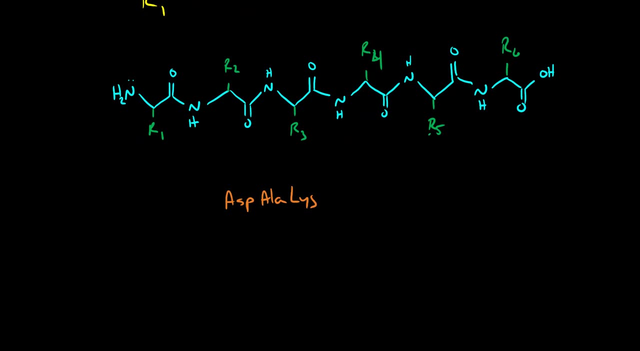 Alla is aspartic, Lys is alanine And Lys is lysine. So we have We call this a trimer, So it's three amino acids linked together. So when we draw this, we're going to want to draw two peptide bonds and then a free. 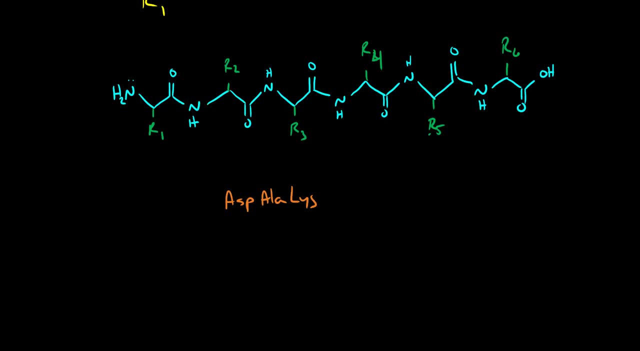 amine and a free carboxylic acid. These are always drawn from the N terminus to the C terminus. So when we draw this we need to have our amine group on the Asp And our carboxylic acid or our C terminus on the lysine. 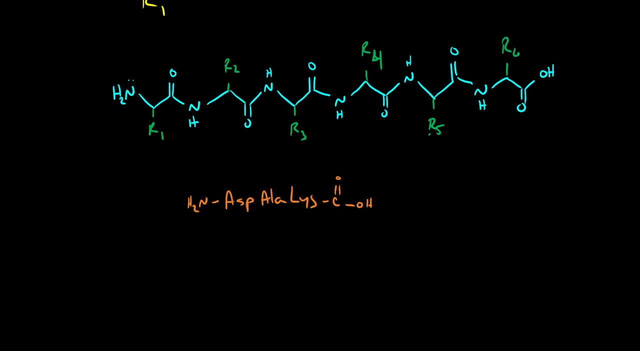 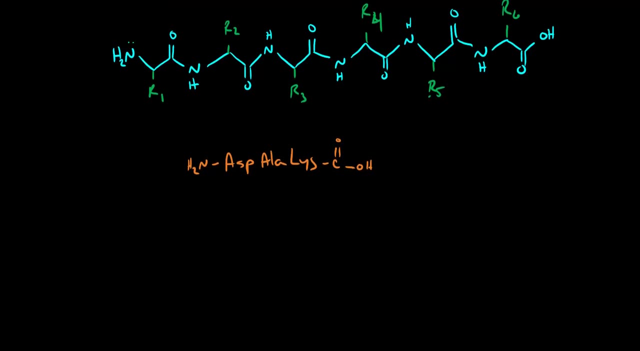 These things are always arranged in this way, From the N terminus, where we have the NH2, to the C terminus, where we have the carboxylic acid. All right, So let's start off by simply drawing in the backbone. 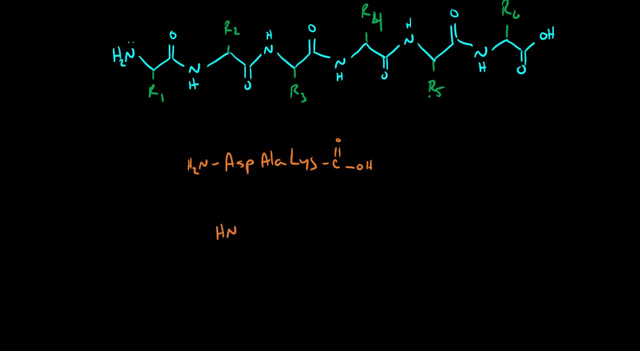 No side chains. yet Start off with your NH2.. NH2, alpha carbon carbonyl, That's the Asp. Nitrogen alpha carbon carbonyl, That's our alanine Nitrogen alpha carbon carbonyl. 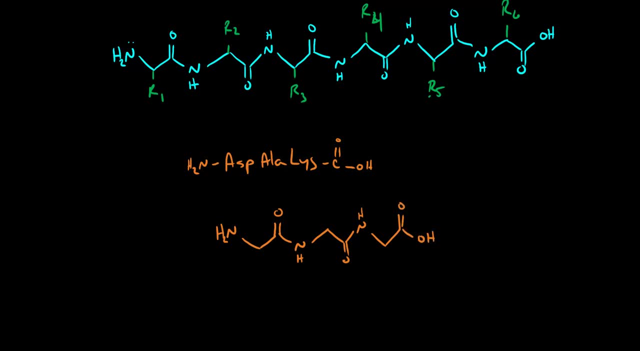 This is the lysine, And now we have our C terminus. This is the backbone. You have to get this right before you can get the overall structure correct, And now it's just a matter of putting in the side chains. Okay, 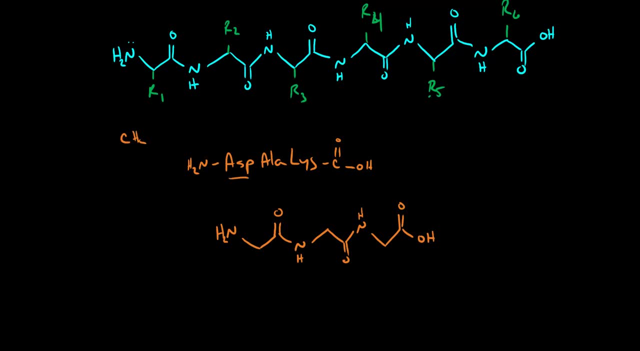 So aspartic acid, you might remember, Aspartic acid is CH2 with a carboxylic acid. Alanine is a CH3. And lysine was the long chain with the amine at the end. So aspartic acid is CH2 with the carboxylic acid. 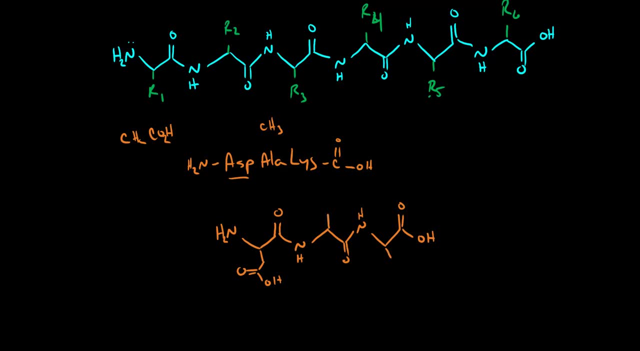 Alanine is a CH3.. Lysine was L-Y-S-I-N, with the nitrogen there. Lysine was L-Y-S-I-N. Lysine was L-Y-S-I-N. Lysine was L-Y-S-I-N.